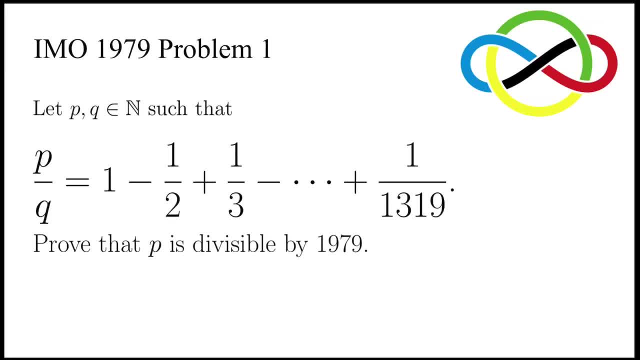 Let's take a look at this problem taken from the International Mathematical Olympiad 1979.. It says: let p and q be natural numbers such that the fraction p over q equals. the given alternating series Prove that p is divisible by 1979.. Before we move on, don't forget to give a. 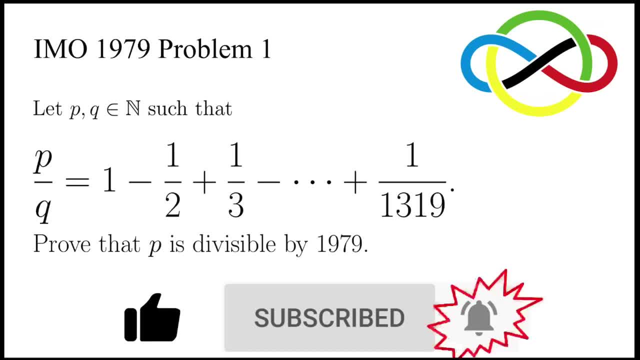 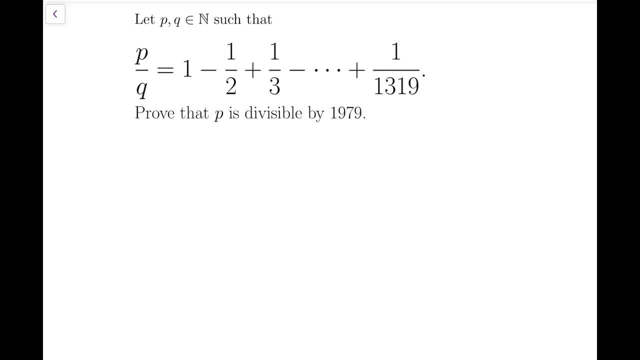 like, subscribe to my channel and turn on post notifications. The weak spot in these kind of alternating series is that all the terms that are that are having the minus sign are fractions, one over some even numbers. So I'm going to rewrite this to regroup the even terms. 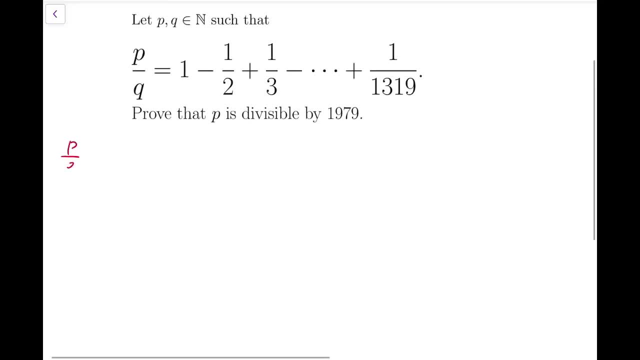 and see what we can obtain. So p over q. by definition is this expression like summing all the odd terms first up to one over one, three, one nine, minus all the even terms up to one over one, three, one, eight. So after regrouping the first half, 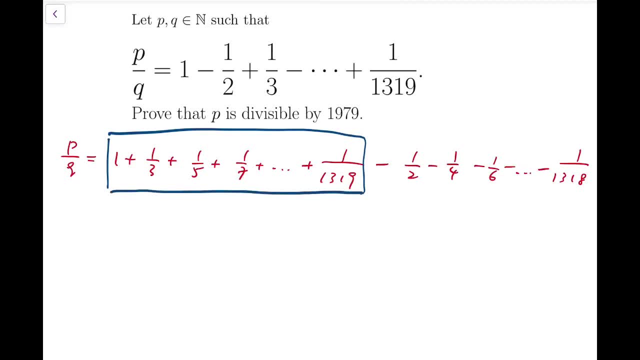 all the adding terms are actually hard to manipulate because it's neither some kind of harmonic series nor it's anything special. So I'm going to add in some even terms to make all the like the denominators to be consecutive. so I'm going to add 1 over 2, 1 over 4. 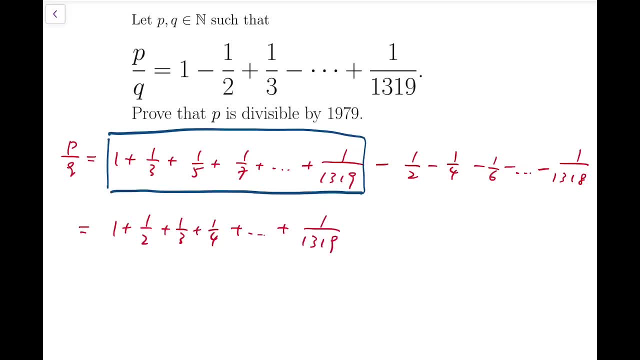 etc. into it, into this, into this part. so it becomes a finite harmonic series: 1 plus 1 over 2, 1 over 3, 1 over 4, all the way to 1 over 1, 3, 1, 9, and then to 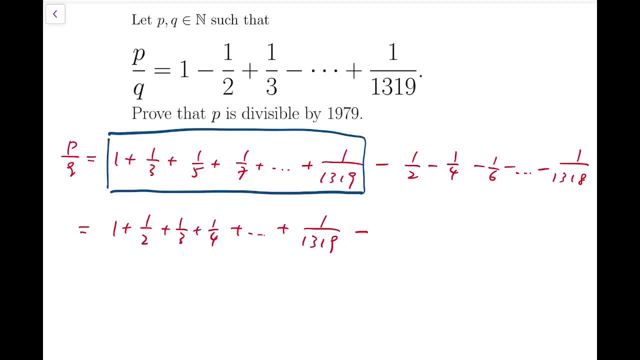 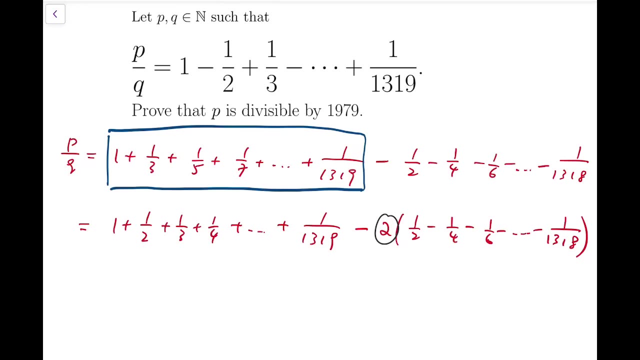 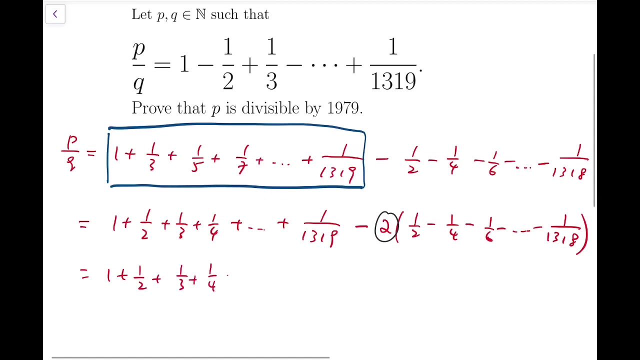 balance the whole whole expression. I need to subtract that back as in I'm going to minus double of the even terms. now, coincidentally, this, this factor of 2, will cancel out with the denominator test, with all the even denominators, and they will become. let me first copy the first half: minus is actually 1 plus. 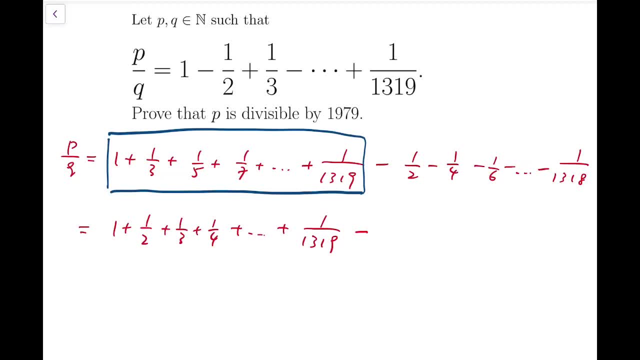 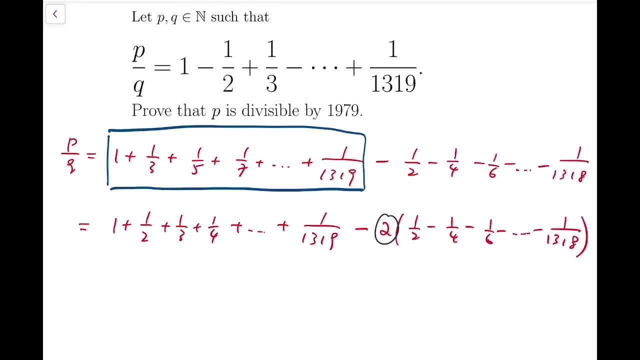 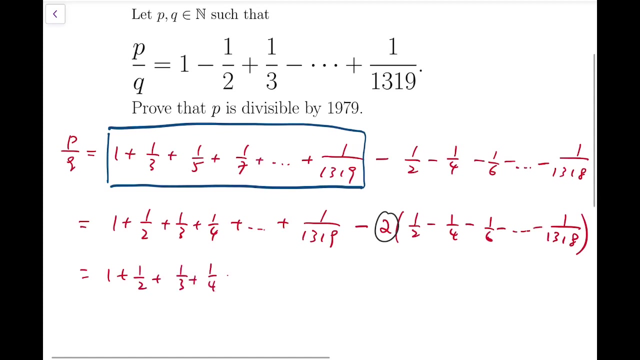 balance the whole whole expression. I need to subtract that back as in I'm going to minus double of the even terms. now, coincidentally, this, this factor of 2, will cancel out with the denominators, with all the even denominators, and it will become- let me first copy the first half: minus is actually 1, plus. there are 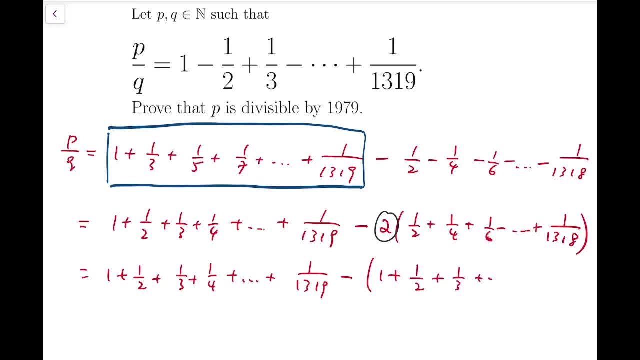 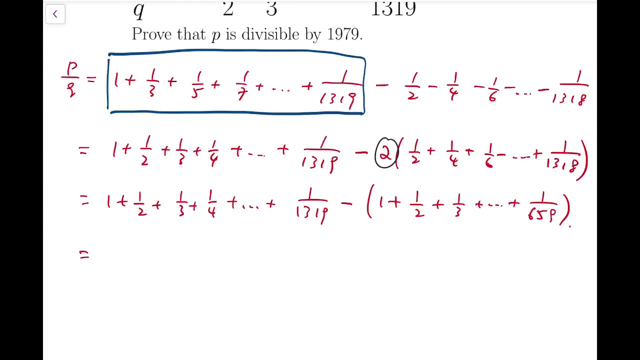 lots of mistakes here: 1 plus 1 over 2, 1 over 3, all the way to 1 over 6, 5, 9. and now I'm. I have two finite harmonic series with me and I'm going to cancel them out. so this: 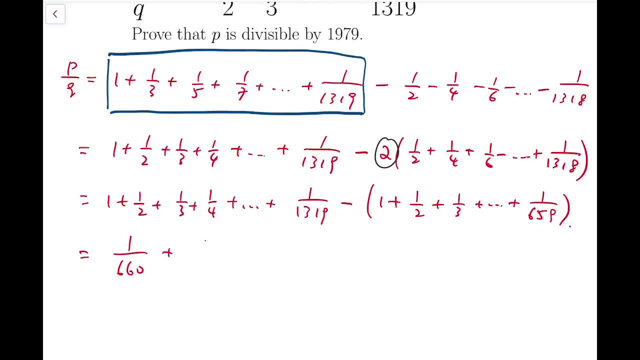 expression now becomes fraction, starting from 1 over 660, 6, 6, 1, all the way up to 1, 3, 1, 8 and 1 3, 1, 9. so this expression looks fine, but we're still quite far from what we have to. 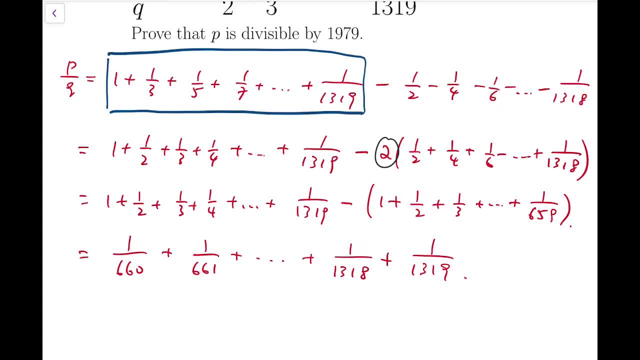 achieve is that we have to be make sure that the numerator is divisible by 1979, this number, but we don't. we couldn't even see the number from our fraction series. so, however, there is actually some way to tackle that, which is to consider the first term and the last term and the second term pair. 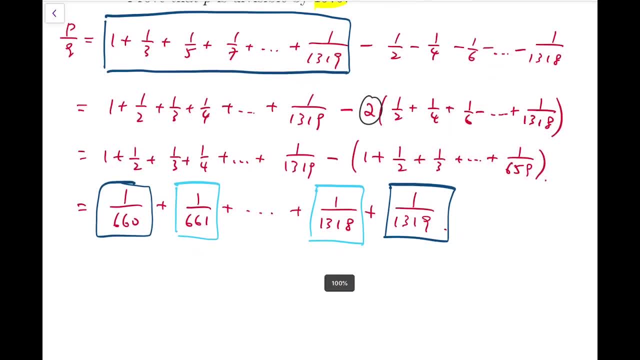 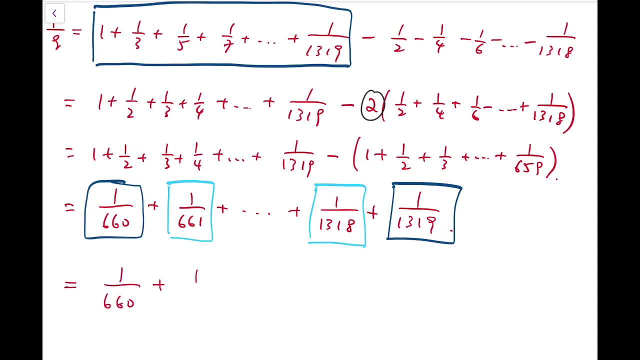 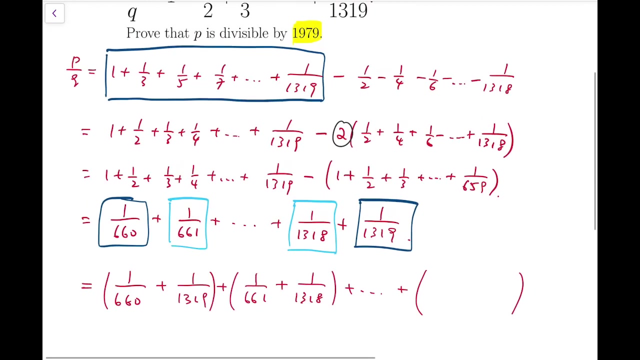 with the second last term, etc. because there's some. if we rearrange it that way, then I'm going to get- if I come to rearrange in this form now this is a bit not regular enough. I'm going to arrange that in kind of in a better way, in fact, for the last 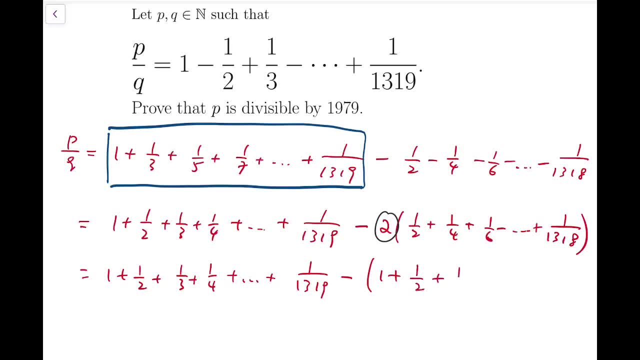 there are lots of mistakes here: 1 plus 1 over 2, 1 over 3,, all the way to 1 over 6,, 5,, 9.. And now I have two finite harmonic series with me and I'm going to cancel them out. 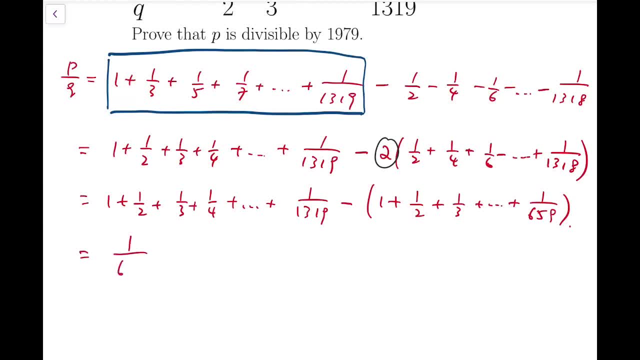 So this expression now becomes fractions starting from 1 over 660,, 6,, 6, 1,, all the way up to 1,, 3,, 1,, 8, and 1,, 3,, 1,, 9.. 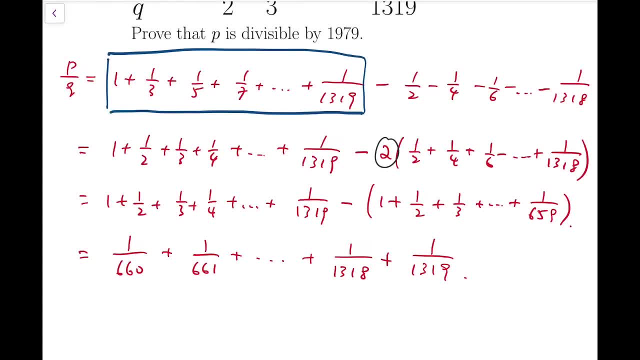 So this expression looks fine, but we're still quite far from. what we have to achieve is that we have to make sure that the numerator is divisible by 1979, this number, But we couldn't even see the number from our fraction series. 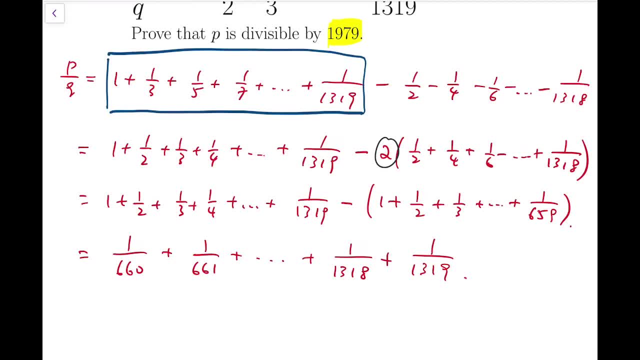 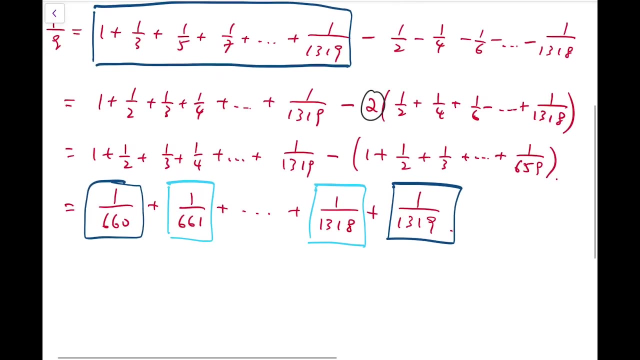 However, there's actually some way to tackle that, Which is to consider the first term and the last term and the second term pairing with the second last term, etc. Because this sum, if we rearrange it that way, then I'm going to get, if I'm going to rearrange in this form, 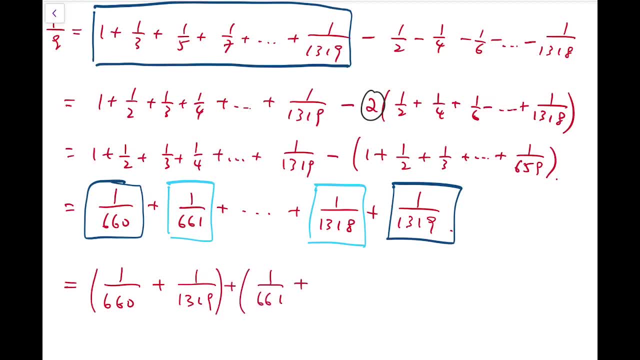 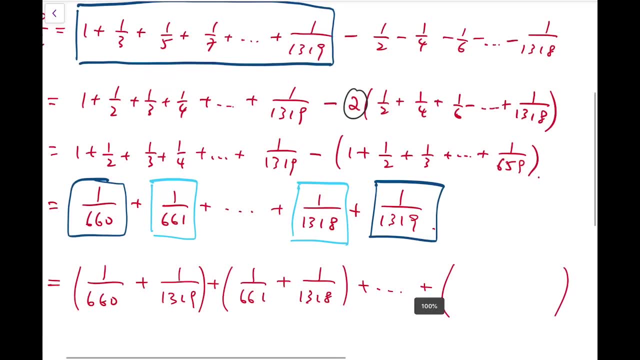 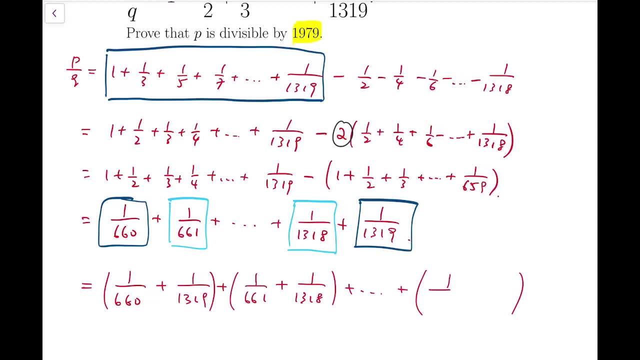 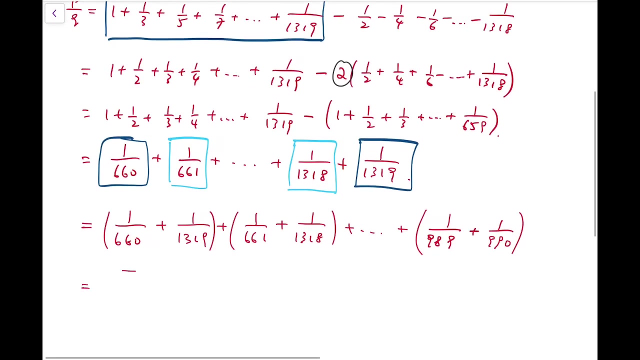 then I'm going to get. now this is a bit not rigorous enough. I'm going to arrange that kind of in a better way, In fact, for the last two terms should be, the last pair should be this: And so I can now rewrite it as a summation: say this all the way to 989.. 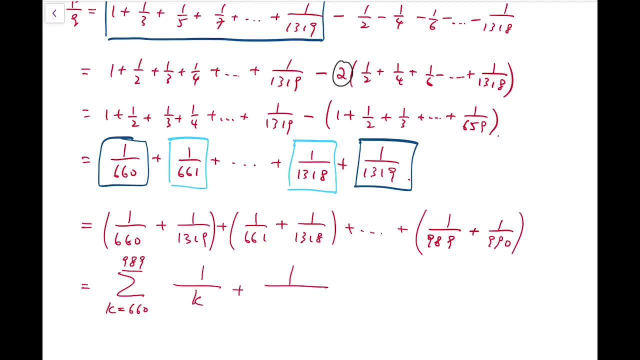 Of the form 1 over, k plus 1 over, and I'll write it as a summation Over k plus 1 over, and I'll write it as a summation all the way to 989.. And in fact the second fraction within the pair is actually 1,979 minus k. 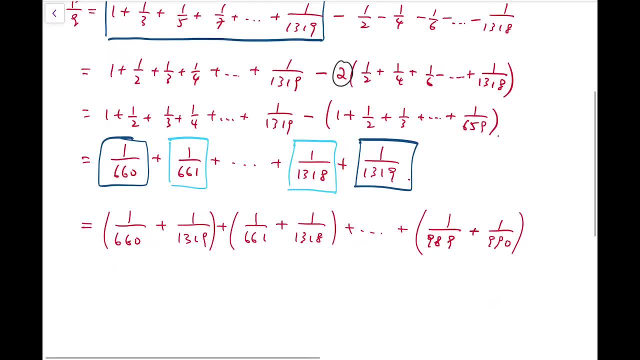 two terms should be. the last pair should be this, and so I can now rewrite it as a summation: say this all the way to 989 of the form 1 over, K plus 1 over, and in fact, the second fraction within the pair is actually 1979 minus K. now, if we 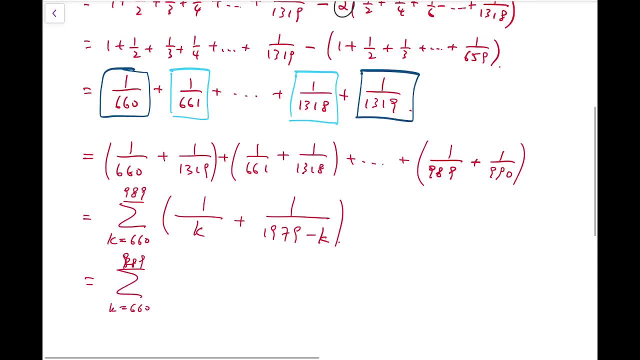 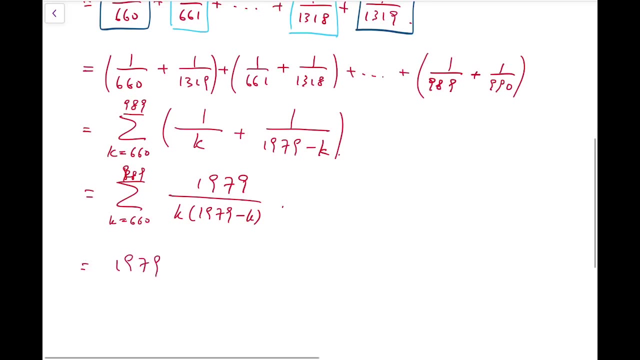 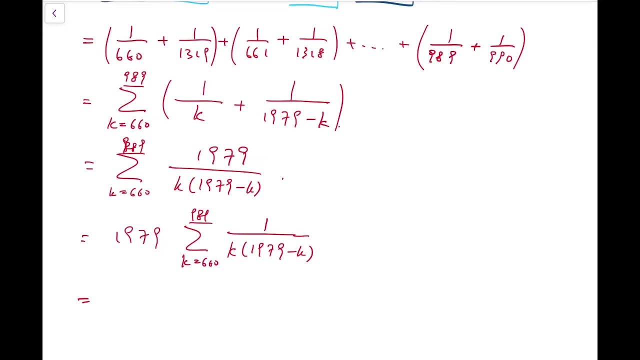 treat it this way, then it will become K times 1979 minus K and numerator is exactly 1979. now I can take out 1979 and and the summation is just another bunch of fractions, one of the form 1 over K times 1, 9, 7, 9 minus K. now if I really do the addition, notice that this number 1. 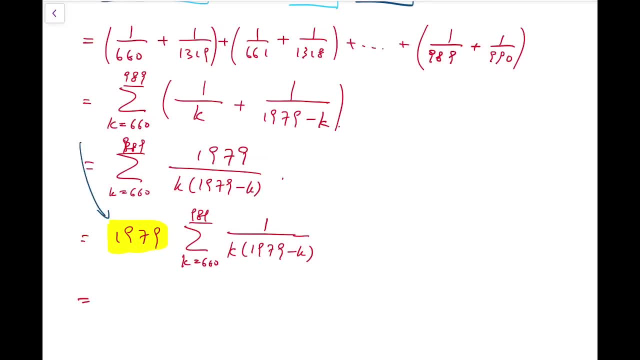 9, 7, 9. this magic number is actually a prime. it's a prime number. so all the terms and the denominator that are of the form K or 1, 9, 7, 9 minus K, ranging K from 6, 6, 0, 0 to 9, 8, 9, they are. they all do not contain the prime factor 1, 9, 7, 9. 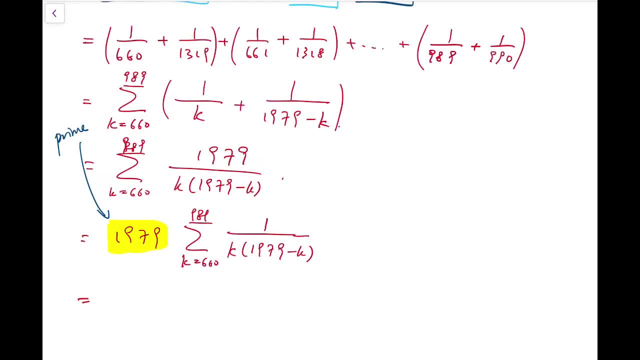 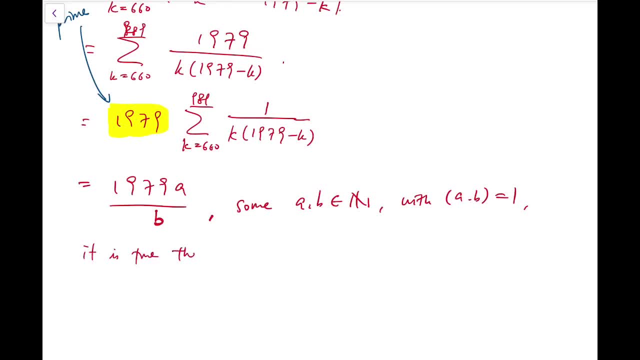 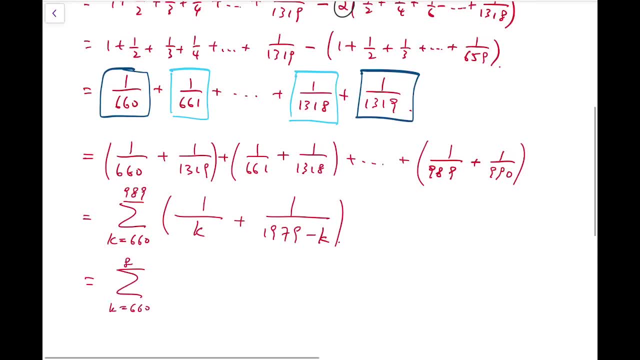 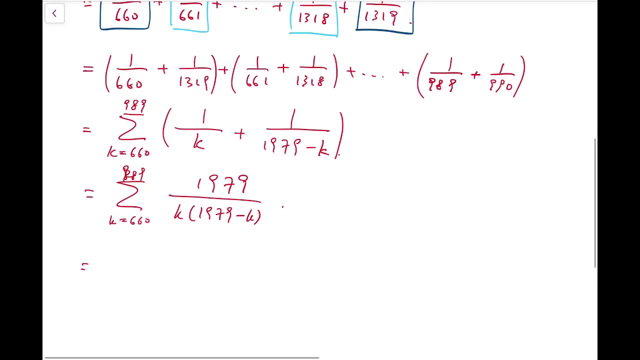 Now, if I treat it this way, then it will become k times 1979 minus k, And the numerator is exactly 1979. Now I can take out the 1979. And the summation is just another bunch of fractions.